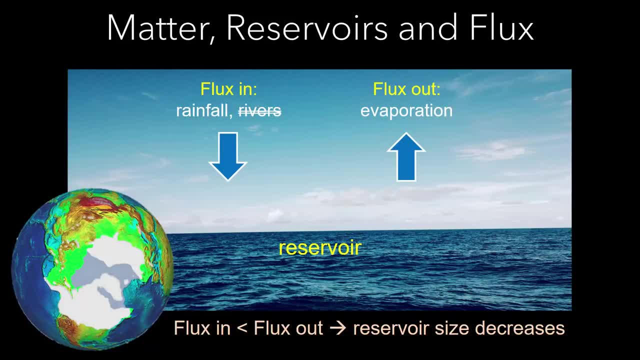 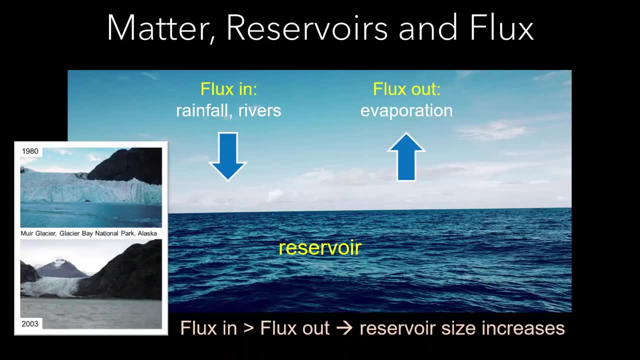 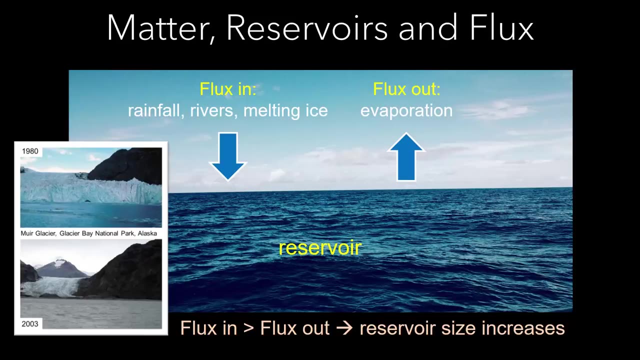 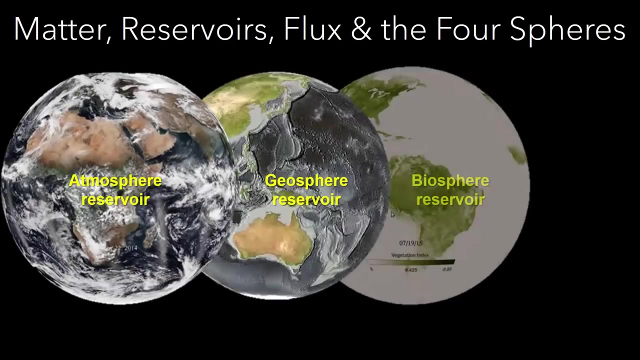 Consequently, sea level dropped significantly, by more than 100 meters. In recent years, the rate of melting of glaciers on the continents has intensified. This has increased flow into the system, producing a larger reservoir and a rise in global sea level. The Earth's system can be characterized by the flow of matter through reservoirs in each of the major spheres. 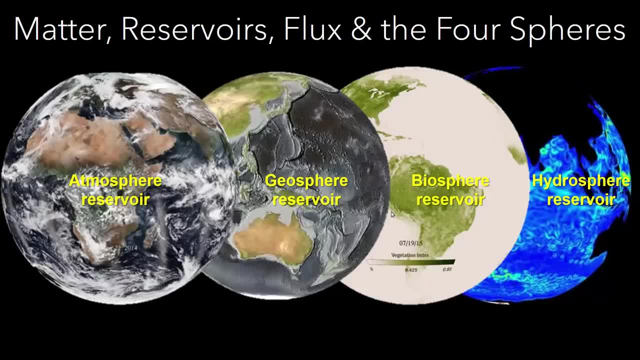 We will describe each part of the system, the relationships between the parts and how those relationships may change over time. To help us do this, we will take a closer look at how different forms of a key element- carbon- moves among the components of the Earth's system. 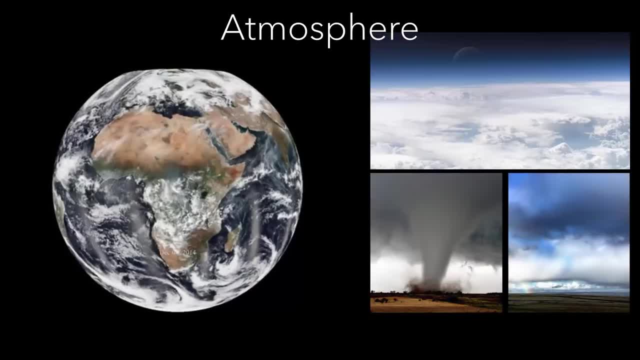 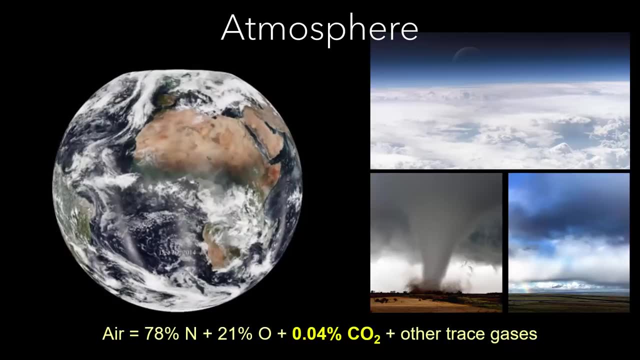 We will start with the atmosphere. We live in the lowest layer of the atmosphere, and this layer contains all the weather that we experience, plus all the air we breathe. The air includes a small fraction of carbon dioxide, along with the more abundant nitrogen and oxygen gases. 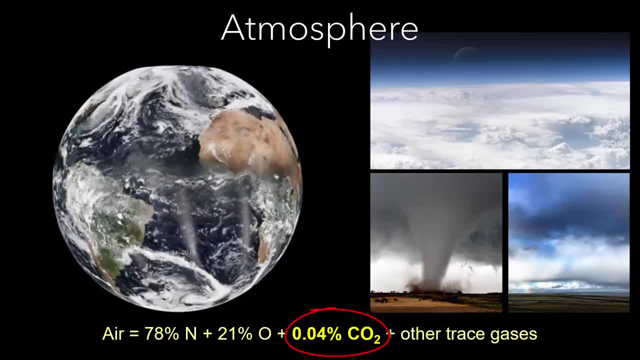 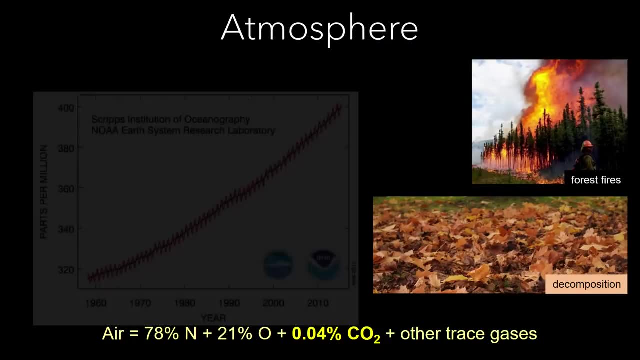 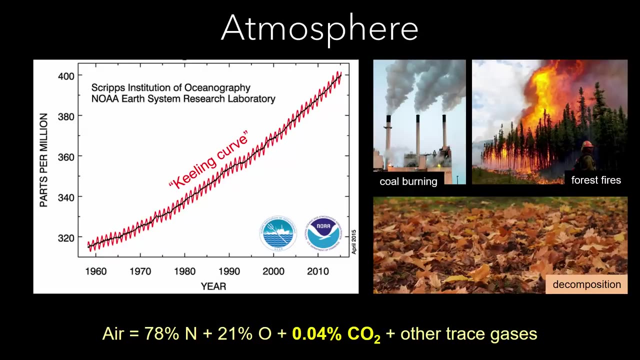 This tiny amount of carbon dioxide makes an outsized contribution to Earth's climate. Carbon dioxide naturally flows into the atmosphere as a result of the decomposition of organic materials and forest fires. The concentration of atmospheric carbon dioxide has increased as a result of the greater use of carbon-rich fossil fuels. 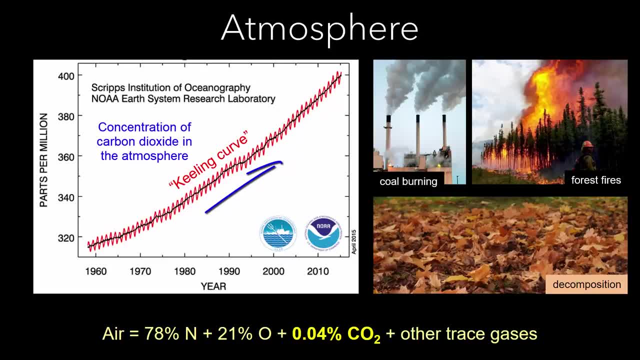 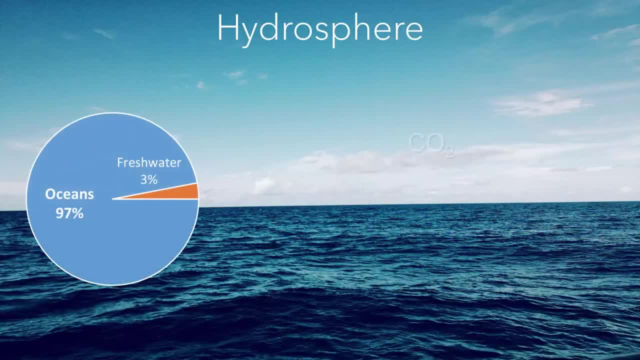 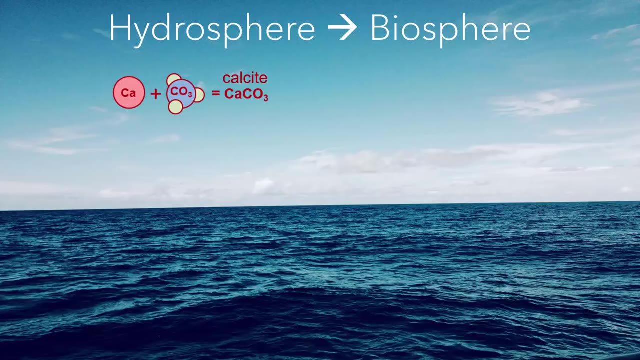 This plot, known as the Keeling curve, records the steady increase of carbon dioxide in the atmosphere. The world's oceans represent the vast majority of the hydrosphere. Carbon dioxide and other gases are exchanged between the atmosphere and the ocean. The carbon becomes part of a carbonate ion that combines with calcium to form the mineral calcite. 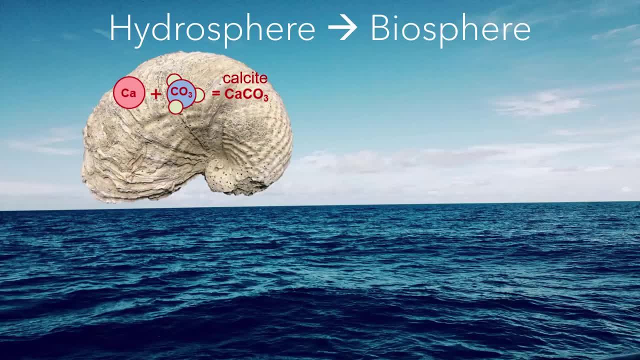 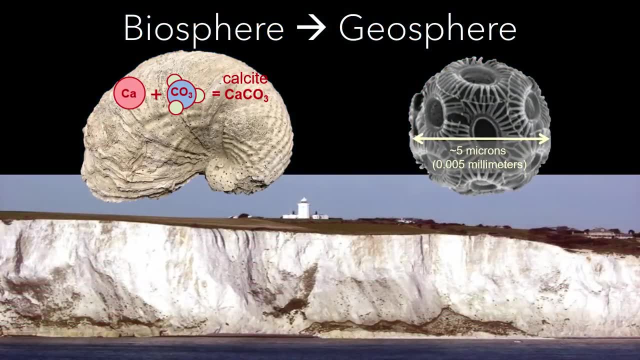 as it becomes part of the biosphere to build shells for things like oysters and clams, as well as billions of microscopic organisms like these coccolithophores. The rock limestone forms when these organisms die and are buried and compacted into layers of rock on the seafloor. 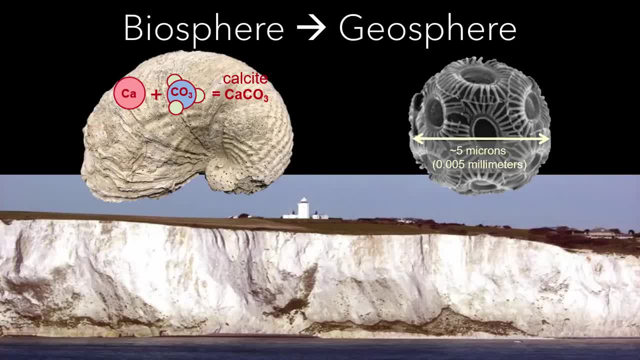 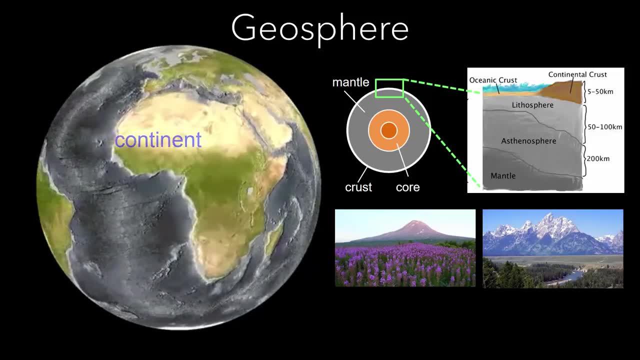 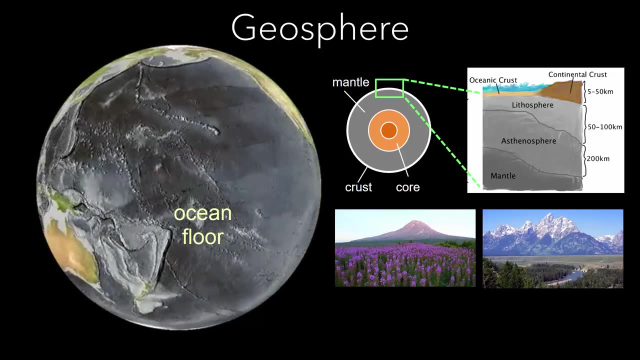 Thus matter moves from the biosphere to the geosphere. The geosphere includes the atmosphere. The geosphere includes the continents and oceans' floors and the rocks and minerals in Earth's crust, mantle and core. Most rocks remain in the geosphere for millions of years, making them part of the Earth's largest carbon reservoir. 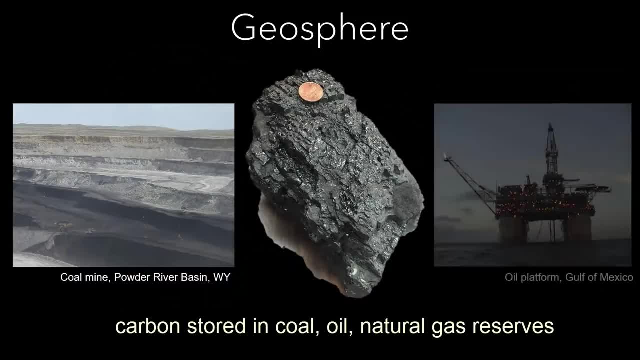 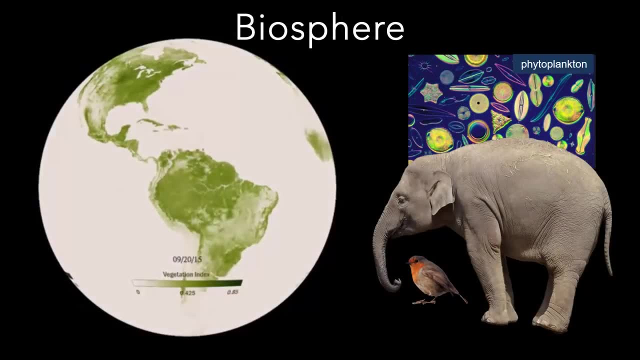 There's more carbon stored in the geosphere's fossil fuel reserves than there is throughout all of Earth's biosphere. The biosphere is composed of all the living organisms on the planet. This is everything from vegetation on the continents to microscopic phytoplankton in the oceans. 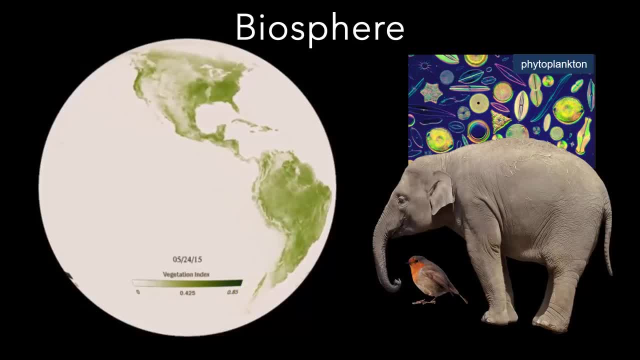 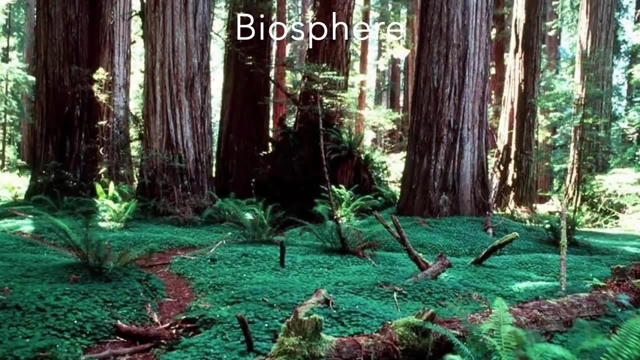 and familiar complex organisms like elephants and birds, And let's not forget humans. Most of the carbon in the biosphere is present as plant material or is found in soils. Plants take in carbon dioxide from the atmosphere through photosynthesis and combine it with other elements to form carbohydrates needed for growth. 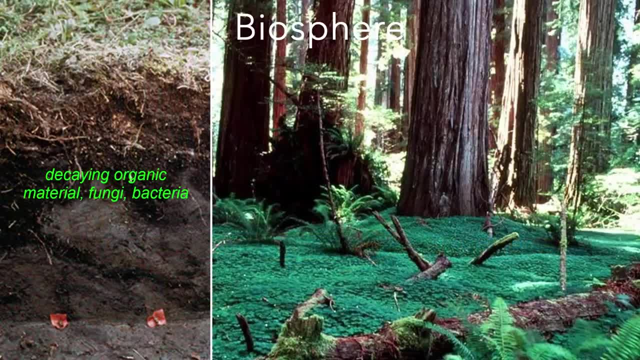 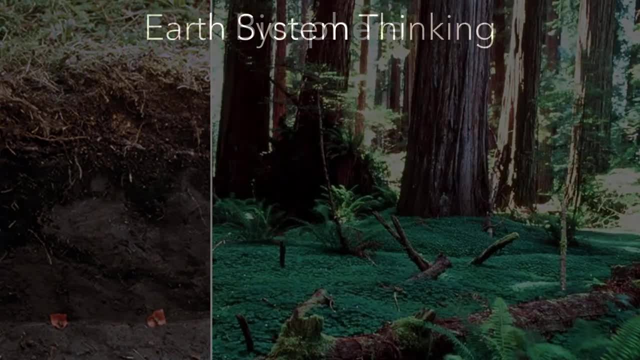 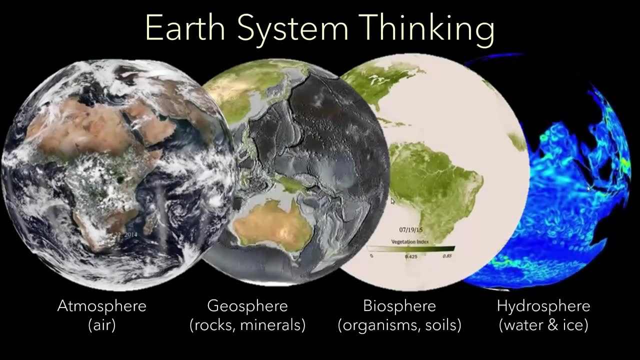 Soils contain more carbon than plants, most of it in the form of decaying plant material and living biomass of microbes that help break down the dead plant matter. So now we know a little bit more about each part of the Earth's system and some of the relationships between the parts. 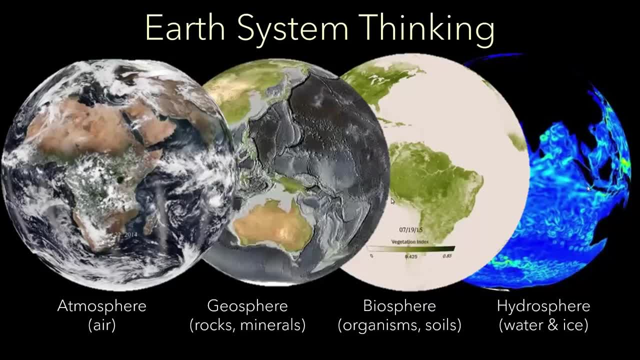 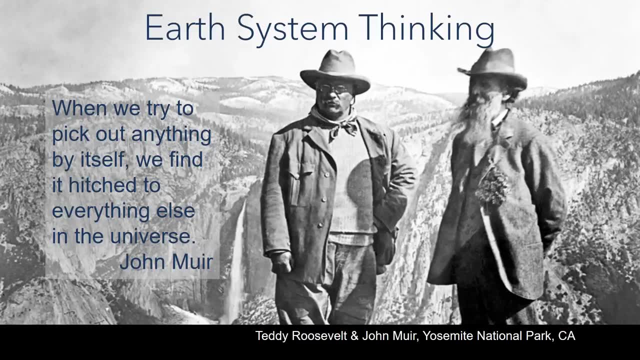 Next we will look at an example of how those relationships change over time. If we want to think more deeply about how the Earth's system works, we might begin by considering a quote by conservationist John Muir. He noted that whenever we try to pick out anything by itself, 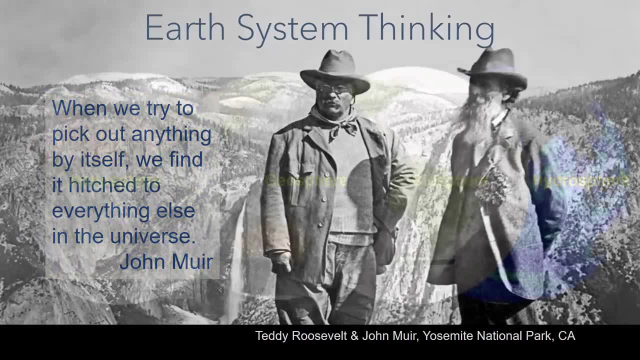 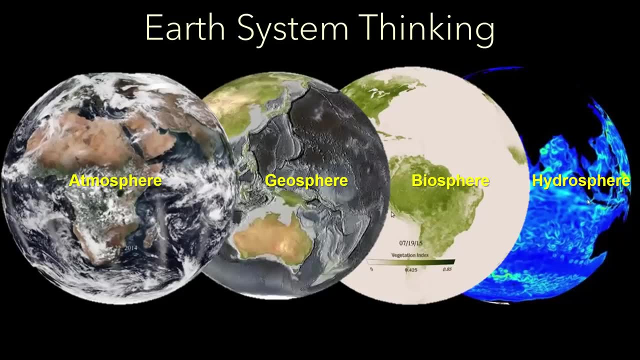 we find it hitched to everything else in the universe, Or to put it in the context of the Earth's system: if we change part of one Earth's system component, it will result in changes in the other parts of the system as well. 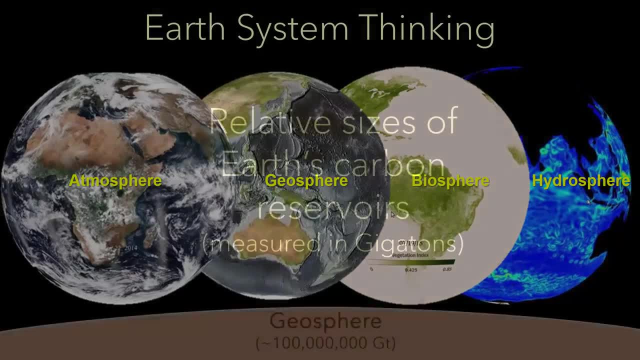 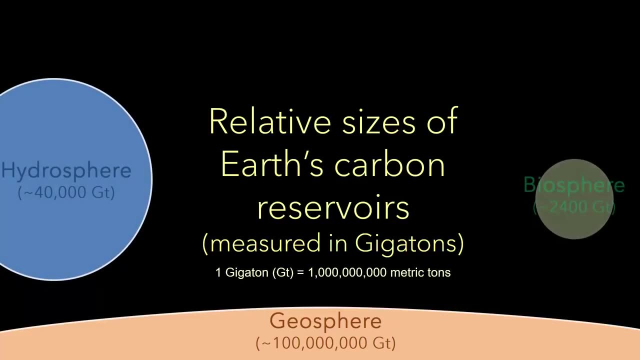 That's exactly what has happened in the case of the world's carbon. This figure shows the relative sizes of the carbon reservoirs within each component of the Earth's system. Note that the geosphere has the largest amount of carbon and the atmosphere has the least. 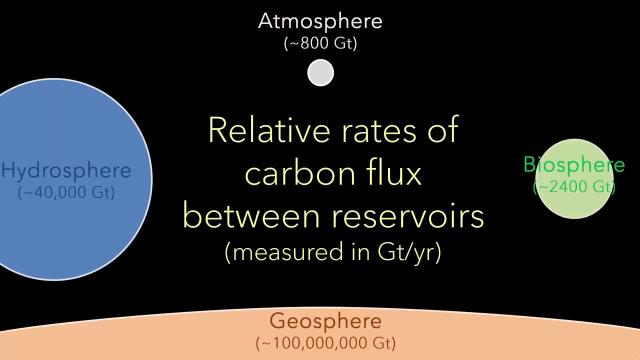 However, while the atmosphere is the smallest of the reservoirs, it experiences the largest relative flux. In contrast, material moves in and out of a natural geosphere reservoir very slowly over millions of years. It's only when human actions perturb this reservoir. 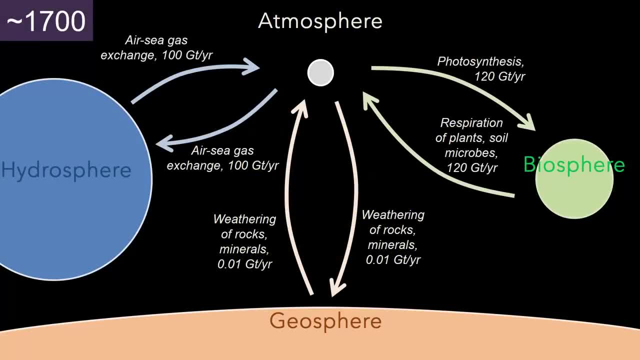 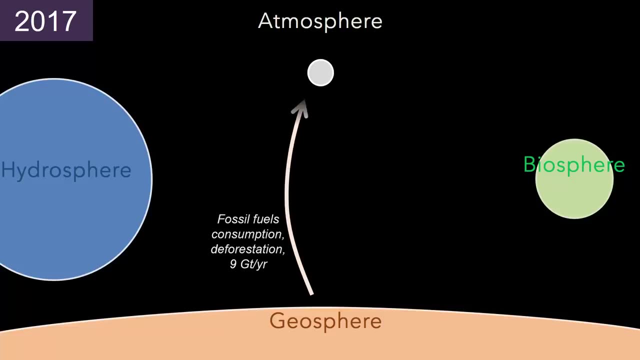 that it experiences more rapid flux. For example, up to a few hundred years ago, the flow of carbon among some of the system components would have looked something like this, with the carbon exchange between the different spheres being relatively similar. However, after the Industrial Revolution,